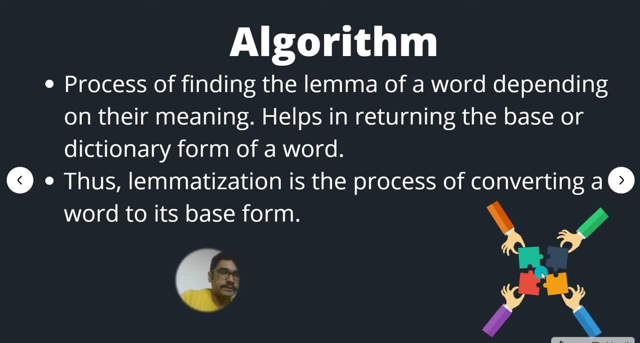 of a word. So, as you can see a small diagram which I've kept on this side, So it's like people are taking small jigsaw puzzles and they are joining. So this diagram can be viewed in two ways. So it can be viewed like people are joining these pieces together or they 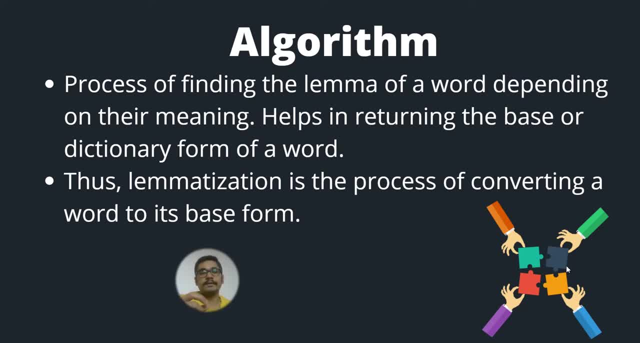 are removing out of this. Okay, so when all the pieces are together, they are removing out of this. So when all the pieces are together, they are removing out of this. So when all the four people join this thing, then it makes a sense. Or if one person is removing or one. 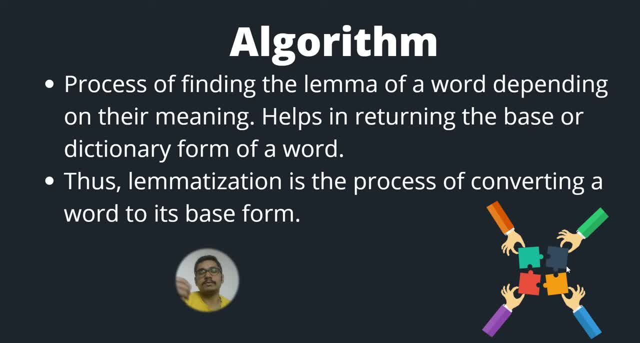 part is missing, then that doesn't convey any sense. So it's where the lemmatization algorithm comes into picture. So thus, as it is rightly said, lemmatization is the process of converting a word into its base form. Okay, so whatever its base is actually, I mean. 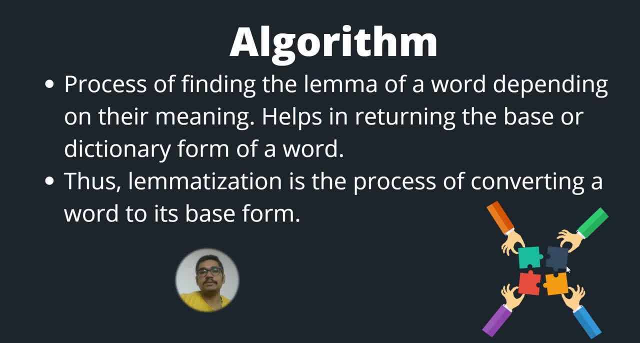 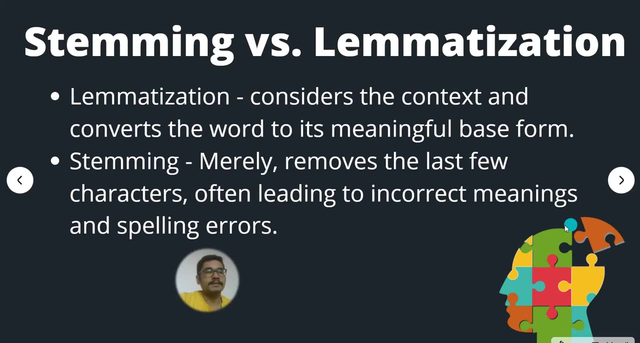 the stem, So that can be easily Understood, or that process can be made more accurate only by using the lemmatization. Okay, so having talked about that, we'll just go on to the difference between what is lemmatization. 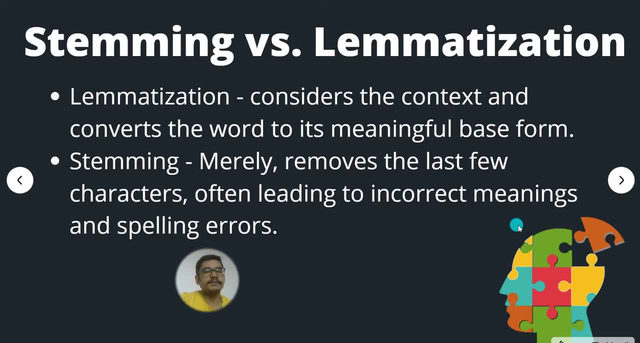 and stemming. So just a small thing, just to keep in mind: lemmatization considers the context and converts the word to its meaningful base form, So it can be considered like a child who is there in a school who doesn't speak something absurd. So he everything answers. 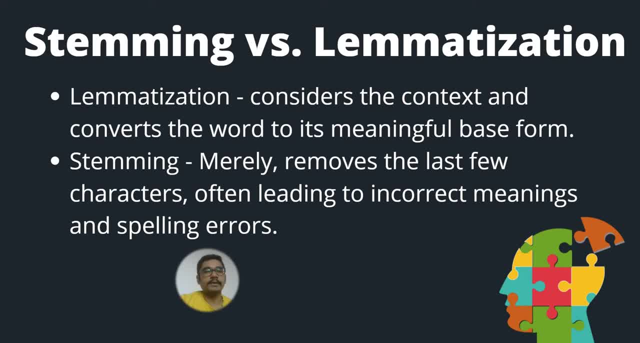 everything dependent upon the context. Okay, and stemming merely is just the opposite. So it removes the last few characters, often leading to incorrect meanings and spelling errors. So if you didn't understand one particular word, then you might miss some words or you might. 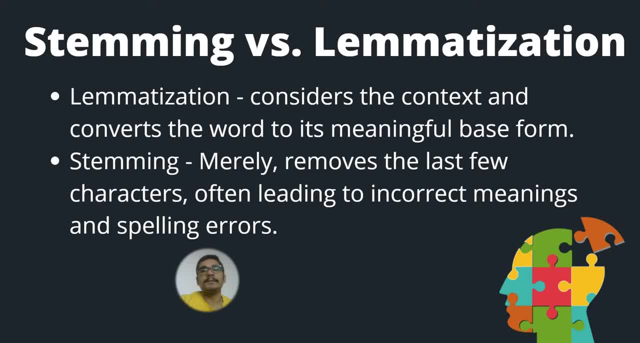 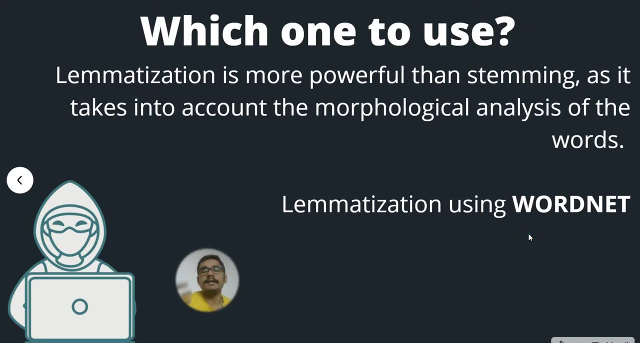 Enable, Engulf some words inside and you'll speak partially about that. Okay, so that is nothing but your stemming. Okay, so the next part is which one to use. So ideally, both should be used, but it highly depends upon the context where you're actually using this. But in a 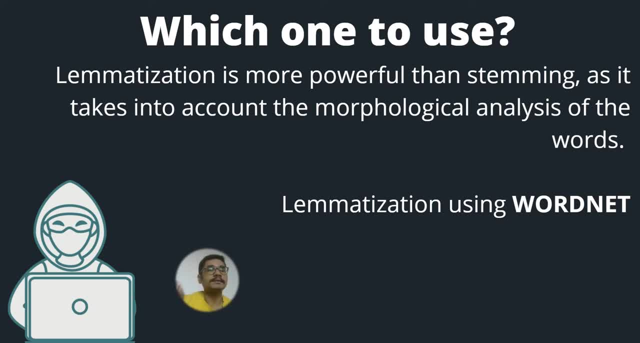 general sense, lemmatization is more powerful than stemming, as it takes into account the morphological analysis of the words. That means how a word is actually formed from its stem and to what context it actually falls into. Okay, so in English language literature you have different words that sound similar. 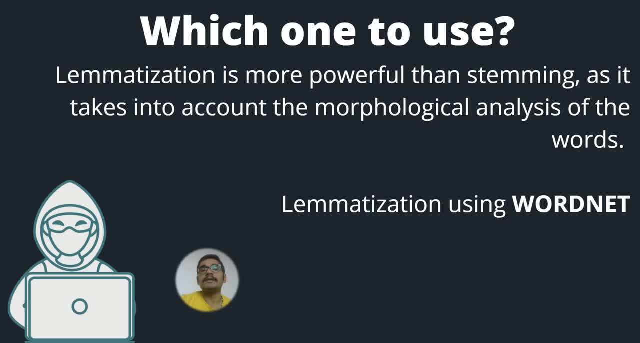 I mean, the tone of the words are similar, but they have different meanings in different contexts. Okay, so in order to be more accurate in those kinds of activities, you have to do the lemmatization first. Okay, so in order to be more accurate in those kinds of activities, you have to do the lemmatization. 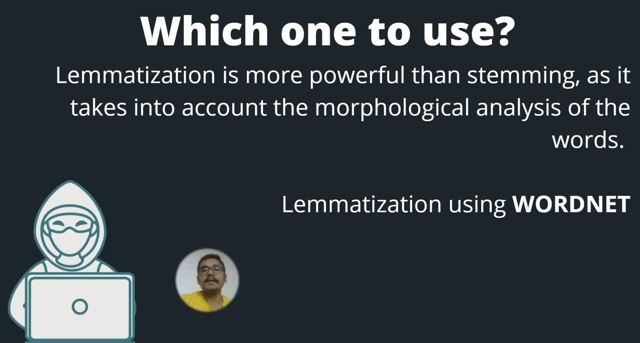 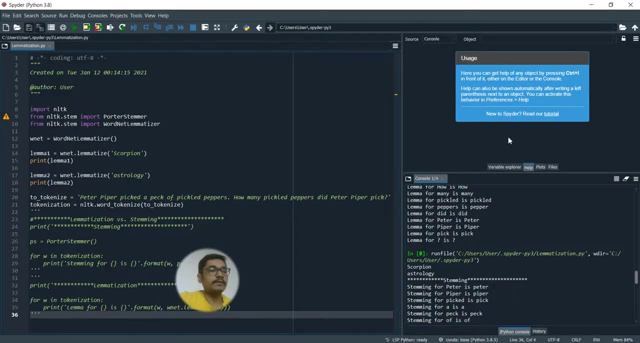 process. Okay, and in NLTK or in NLP, we can make use of the WordNet function in order to make the lemmatization process happen. and now let's quickly move on to the code counterpart. how it looks like. Okay, so this is the code for that. 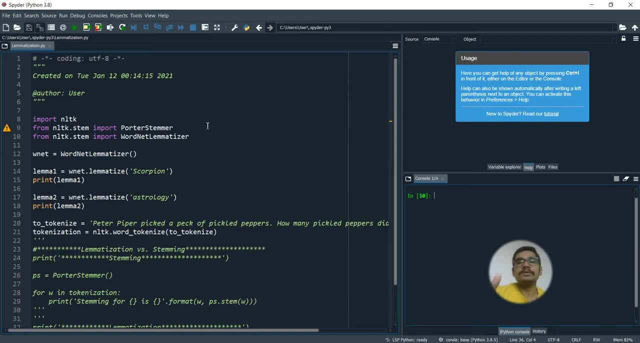 So I am importing NLTK and for doing stemming you actually need any one stemmer algorithm. So we already saw there were three stemming algorithms: porter stemmer, then PS2 was there and you had the Lancaster, and we saw the differences also. So here, just for simplicity, I am taking the very simple stemmer, that is, the porter stemmer. 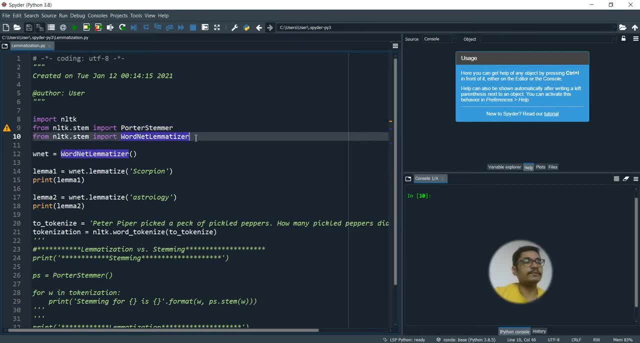 and for lemmatization you have to use the WordNet lemmatizer, So that is the bystander lemmatizer which is present in NLTK library. So first I am making an object of this particular class, WordNet lemmatizer, as WNET. 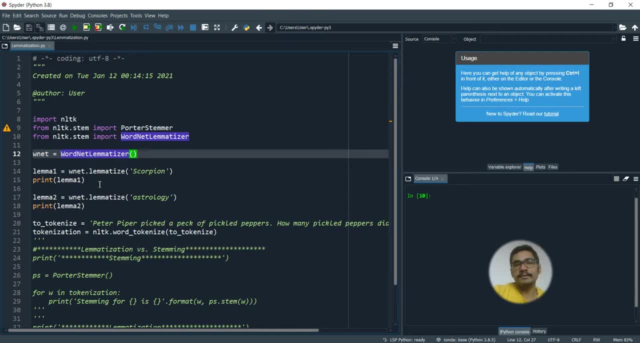 and then I will have two simple examples, that is, two print statements, just to make sure, like it is not changing the meaning of the word or whatever input you have given, it will give out the output as it is. So I have one lemma where I am lemmatizing. 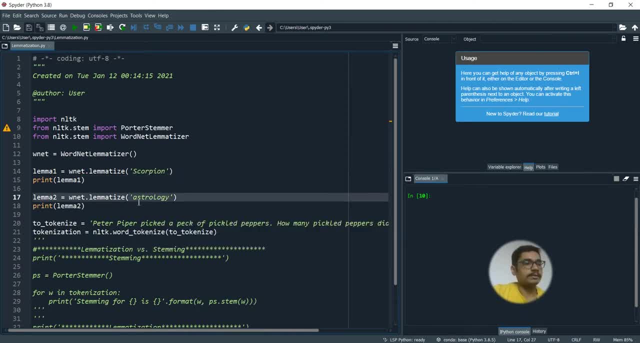 I am lemmatizing a word, scorpion, and the second one is astrology, So if I run this you can see it gave out the word as it is. So there is no difference, or actually you are not doing stemming but the word. actually it is given out, which actually has a meaning in the English dictionary. 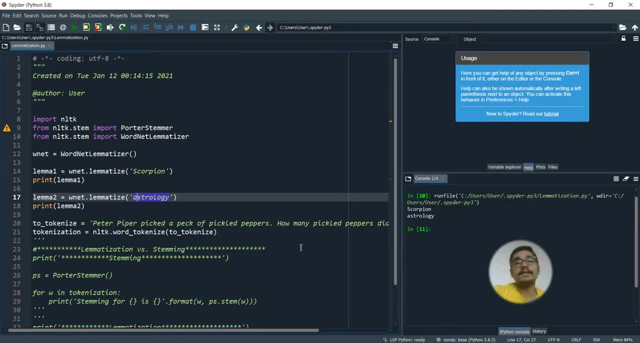 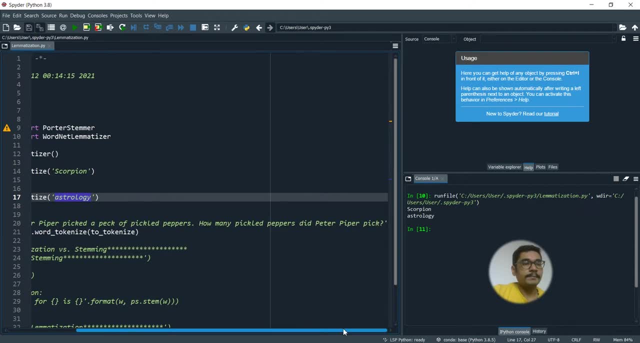 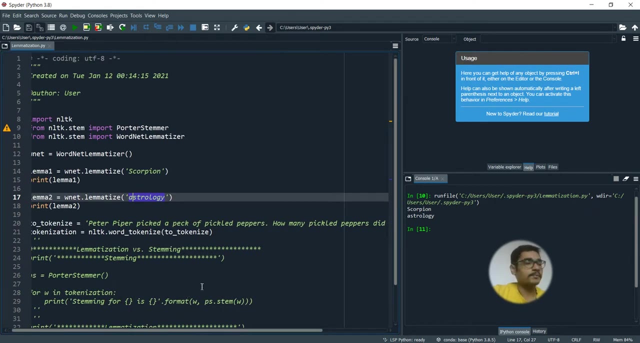 So instead of that, instead of giving tokens, what I will be giving is I will be giving a tongue twister. So Peter Piper picked the peck of pickled peppers. How many, How many pickled peppers did Peter Piper pick? So it is difficult for me also, but we will give it to NLP to do the process. 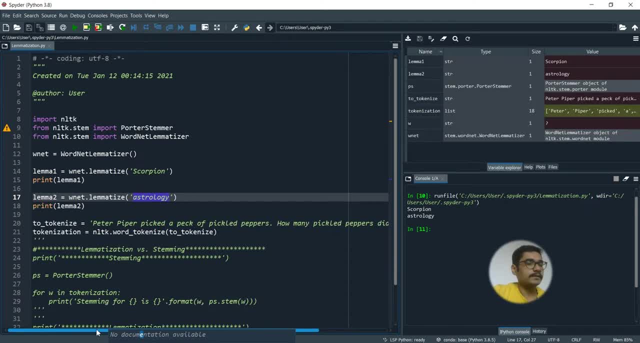 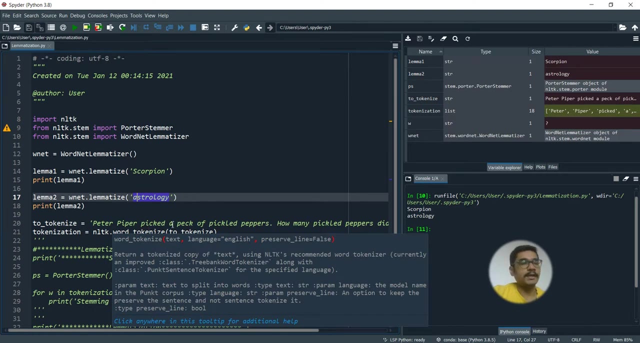 So that particular string is just for tokenization or we are intended to do the tokenization for that. So to tokenize goes into word tokenize, So that is the method that we used to split that particular string into, So tokenization continues. Tokenization contains a list of all the tokens of this particular entire string. 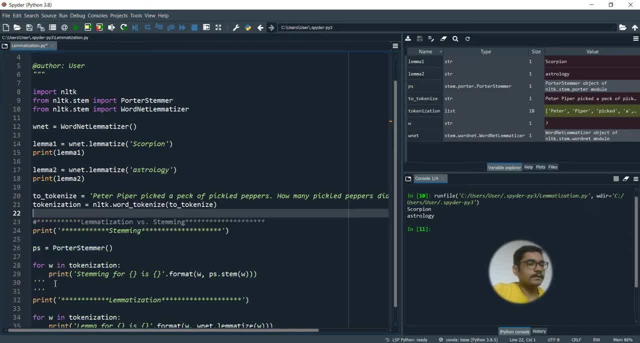 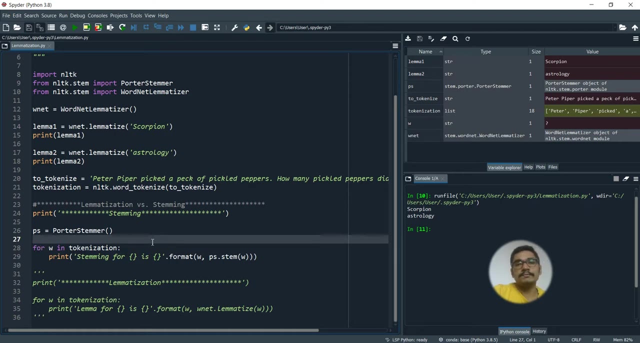 Now, this is just to demonstrate the working of stemming, how it actually works for this entire particular string. So I am creating an object of the Porter stemmer and just a small for loop just for printing all the individual words. And this is just a small for loop. 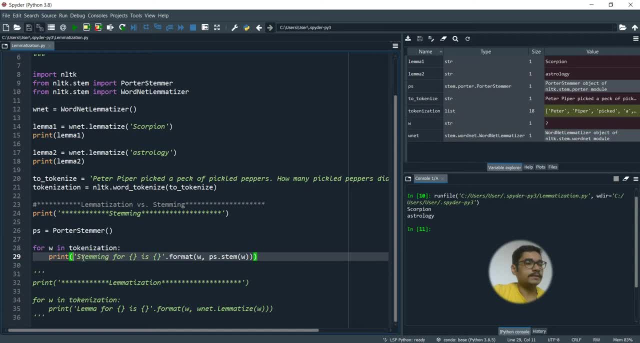 Just for printing all the individual words And they are stems. So that is just by simple replacement operator. we already know, and the stemming actually happens at this process. So this curly bracket will give you the resultant of that, I mean the stem of that particular word. 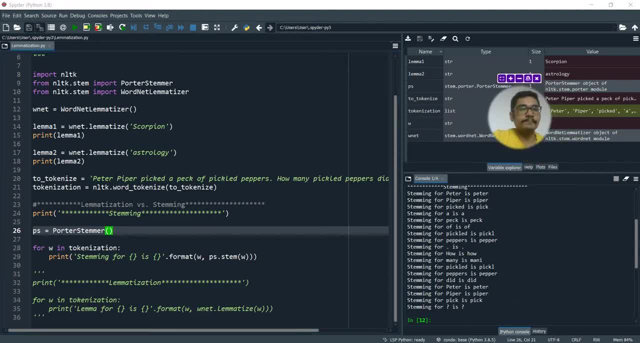 So I will just run this So, as you can see, it gave out the resultant of the stemming. So stemming for Peter is Peter, So it just converted everything to Peter To lower case. then Piper is Piper. pick this pick, So you can see accurately, just trimmed off the root. 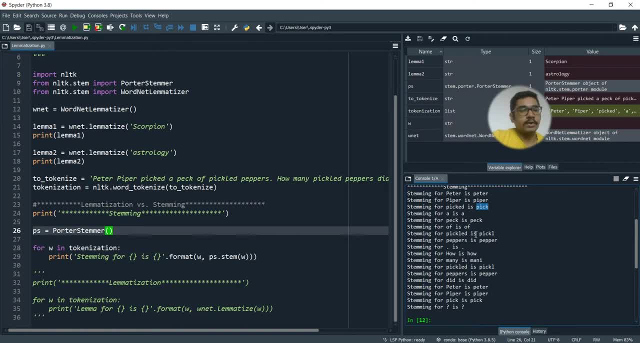 Then A is A Peck, is Peck off, is off pickled is now here. it is not correct. It should be P-I-C-K-L-E: pickle, Then peppers. This is correct. Then That is period operator, I mean the period. 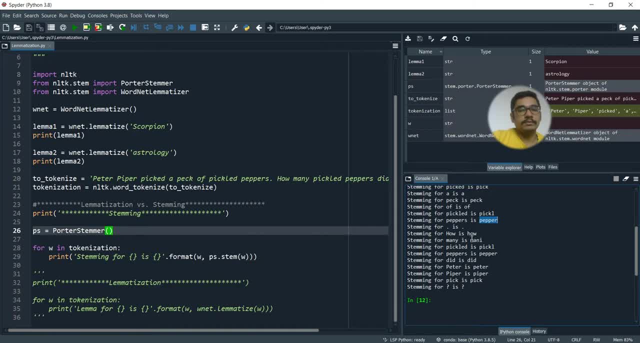 How is how it converted to lower case? Then many, many. it is converted to something: money, So M-A-N-I. So that's not correct. Pickled is P-I-C-K-L, that is again incorrect. Peppers: it has converted to pepper. 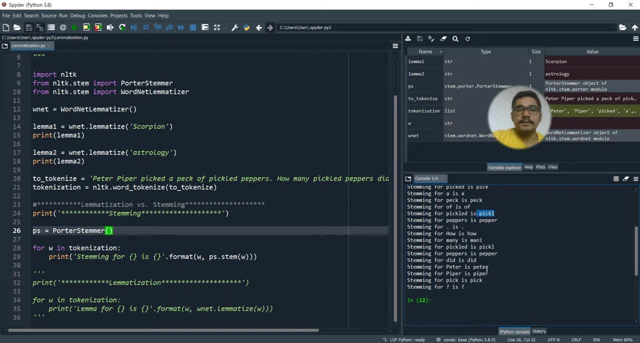 Correct: Did is did. Correct: Peter is Peter. Correct: Piper: Piper Pick is pick, Pick is pick Correct. And question mark: That is for punctuations. It will not do anything for punctuations, Just for word, because we are operating that thing on a complete word. 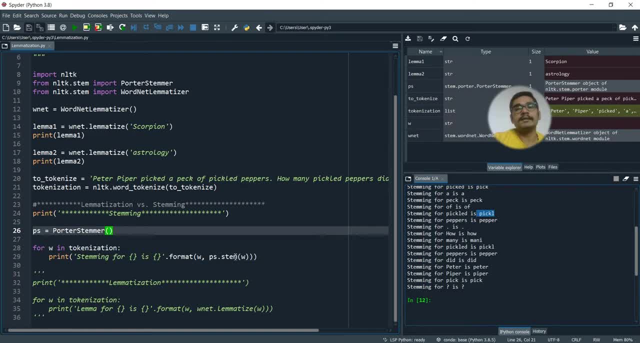 So punctuations won't come into picture. Punctuations are actually your stop words, So that will actually filter out for our process. But this is just for the demonstration of the stemming. Now let's look on to what the lemmatization process has to do. 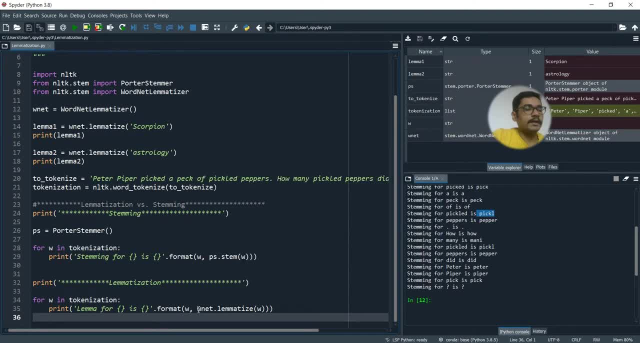 So on the same thing, I'll do the lemmatization. So I'll just use the wnet object from this wordnet lemmatizer class and I'll just call the lemmatize function over the stem function and we'll just look for the code, what it is. 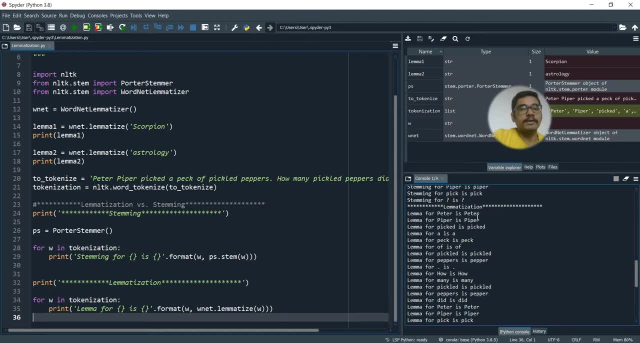 So we have already seen the stemming output. Now this is the lemmatization output. So, as you can see, pickled is. it's kept as pickled. Okay, The input was pickled, But the lemmatization process converted to pickled. 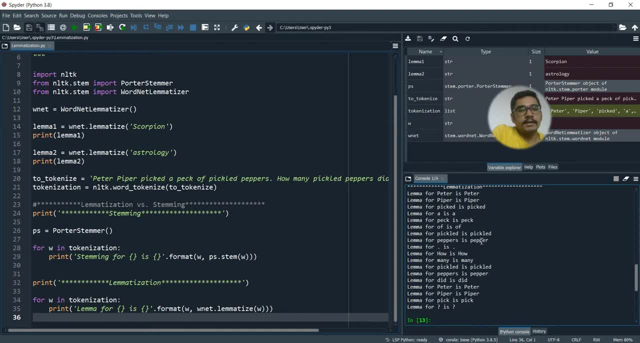 Then you can't make out any mistakes because it's perfect, because everything seems to be perfect as compared to lemmatization, though that's why it is called as more powerful as compared to stemming, because in stemming you have three different algorithms, So they have different behaviors when you give different data sets. 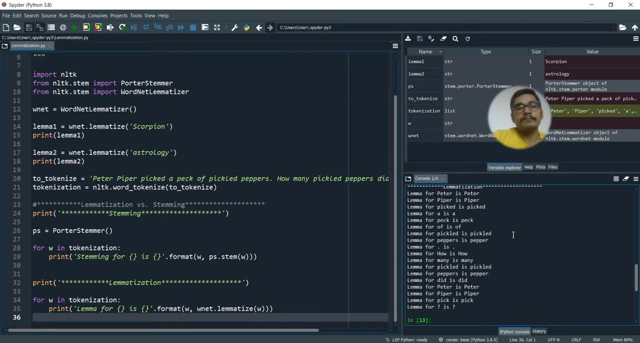 So it will work accordingly dynamically, but in lemmatization it's not like that, just a standard process for lemmatization for different tokens and for different strings. So well, that was all regarding a quick overview or introduction of lemmatization in NLP.